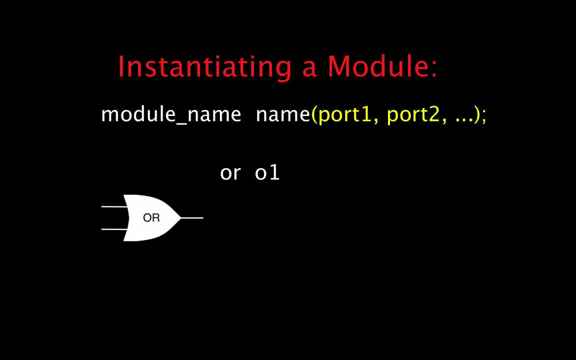 I'll use O1.. To connect the ports I need to know how they are ordered in the module's definition. Verilog's built-in modules follow the conditions of the module, So the output port is first, followed by the input ports. 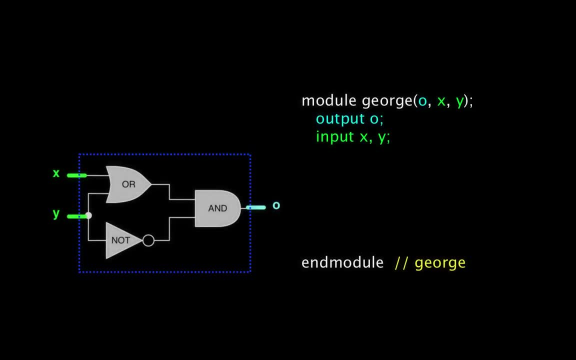 So let's see how to connect this OR gate up in our circuit. We instantiate it in our module and we see that its inputs connect to our two input ports, X and Y. So we write X and Y in the input port. definition of our OR gate. 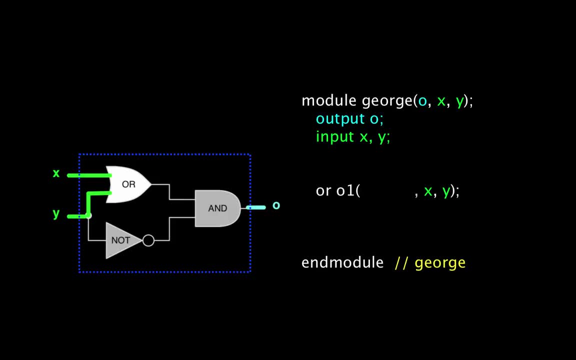 indicating that the OR gate's inputs are connected by wires to our module's inputs, But our OR gate's output connects directly to our AND gate, which is the AND gate. To handle this, we need to declare a wire For our module. we need to declare two wires, which I'll call OR wire and NOT wire. 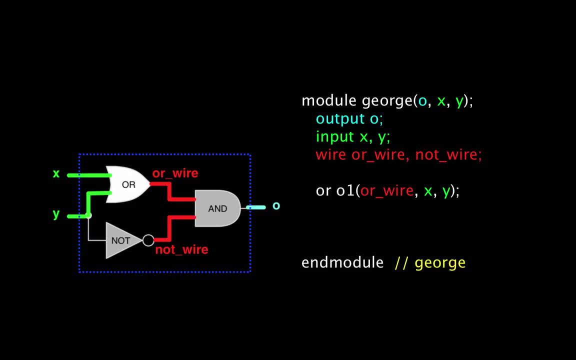 Now I can connect the OR gate's output to OR wire. Similarly, I can instantiate the NOT gate and connect its input to Y and its output to NOT wire. Lastly, I can instantiate an AND gate, connect its inputs and connect its output to the output port O. 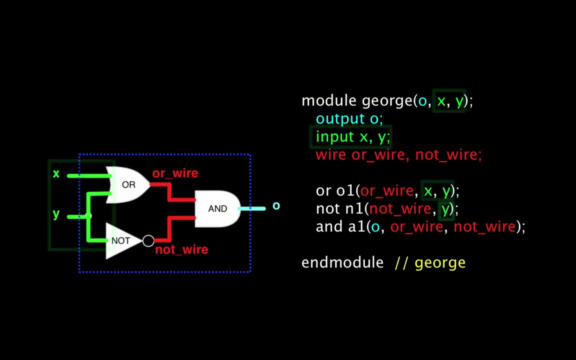 So you can see there is a clear correspondence between the Verilog I wrote and the circuit, And this is how you should think about Verilog: that it is a textual way to describe a circuit and not as a program to run. Let me further clarify two common misconceptions. 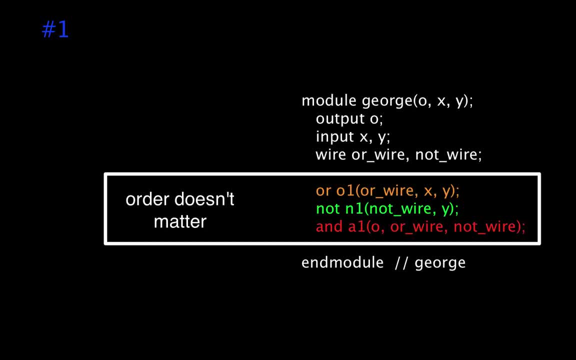 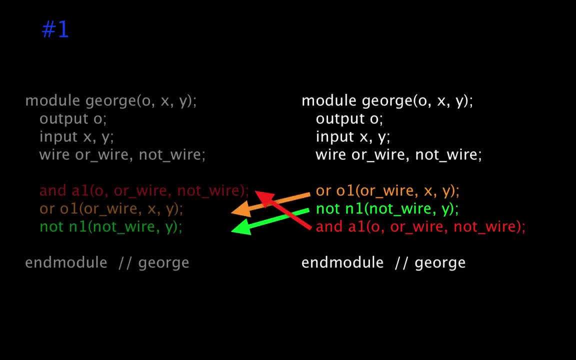 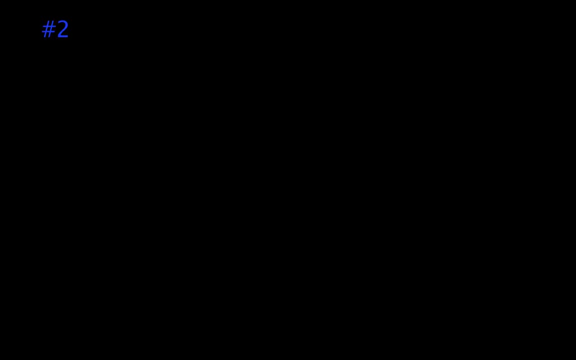 First, the order that we instantiate modules doesn't matter. Our module instantiations just describe how things are connected so we can change their order in the file without changing the topology. Second, students that are used to normal sequential programming are comfortable with reusing variables. 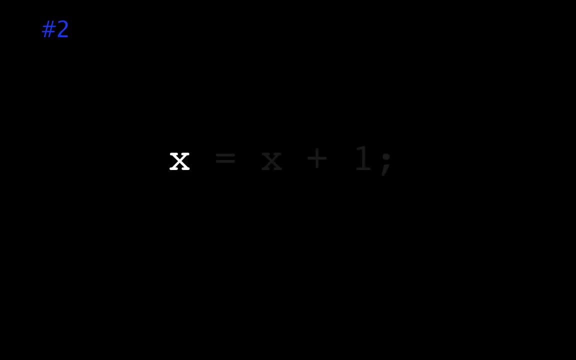 For example, in many languages I can add one to a variable with the following statement: This tragically leads some students to try to reuse wire names, thinking that it would create a circuit like the one shown. But Verilog will connect all module ports with the same wire name within a module.